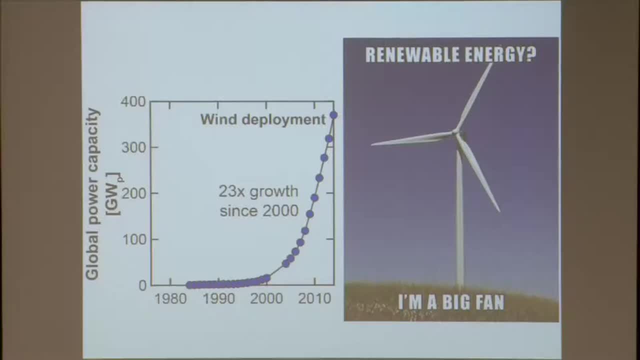 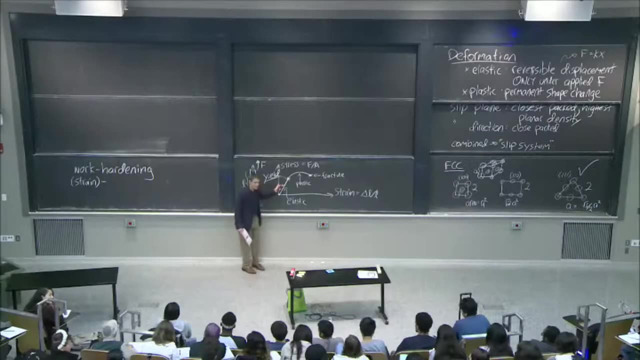 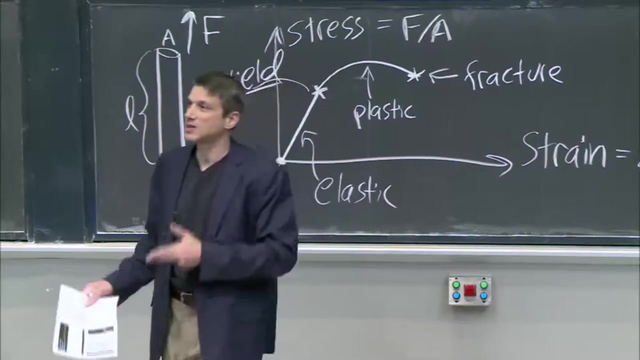 And then how do they need to be strong? Because you've got huge amounts of wind coming at them and it turns out you need to hit just the right balance of elastic deformation before it goes into some plastic regime. You need to hit just the right balance of ductility. 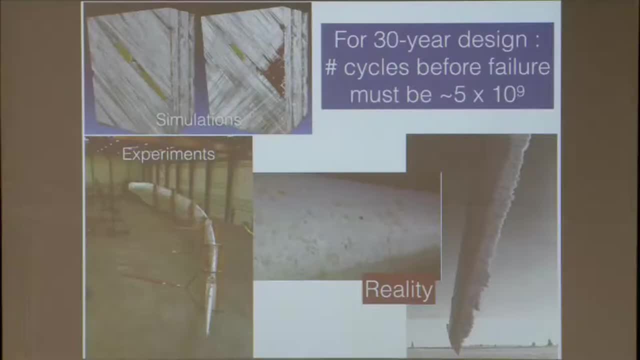 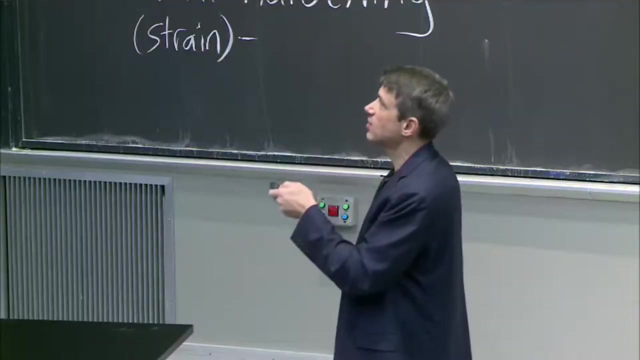 So here's, for example, these are some simulations, Here are some experiments on a new material for a wind turbine blade, And then you put it out there and look at what happens- Ice, By the way. this ice comes off at hundreds of miles an hour in chunks. These farmers, 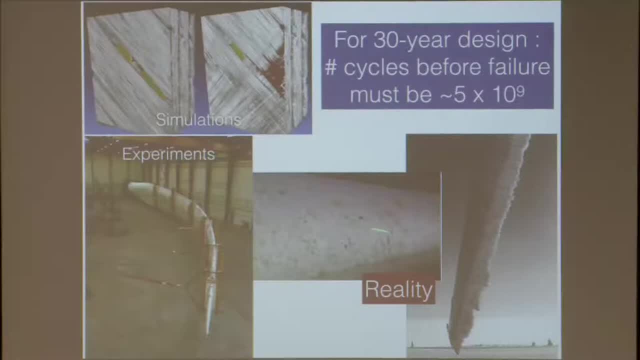 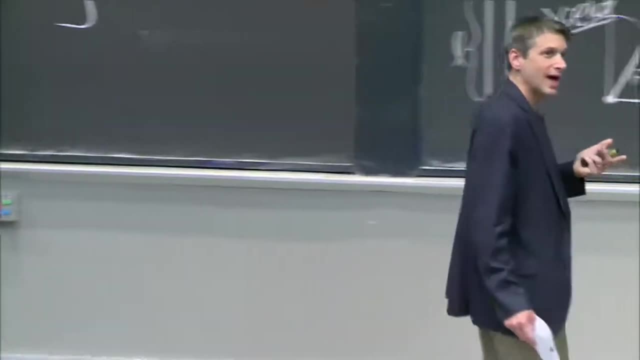 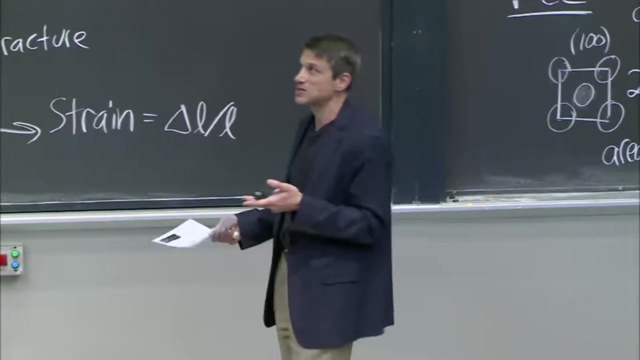 are not happy about that Seriously, But those are bugs, Those are bugs. So actually bugs in wind turbine blades is a serious problem. How do you clean bugs on off of it? because it dramatically changes the aerodynamics and the efficiency. It also can damage the blade itself. 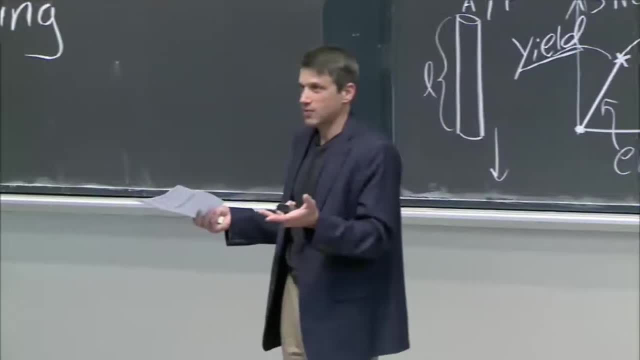 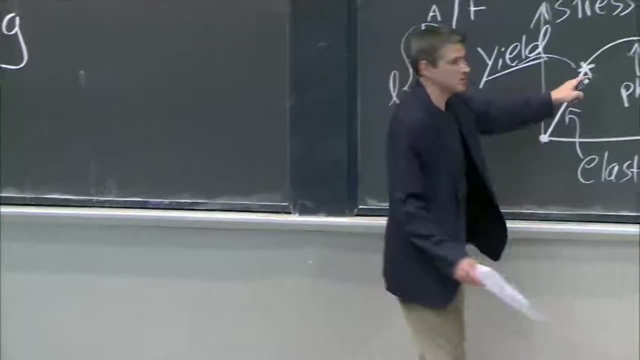 So there's all sorts of work going on. How do you make bug-proof wind turbine blades? OK, we'll now just spray it with something. Ah, but then does it have the right plastic. different What? does it have the right yield point? 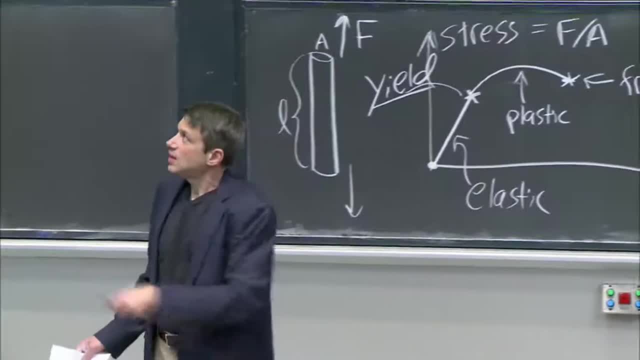 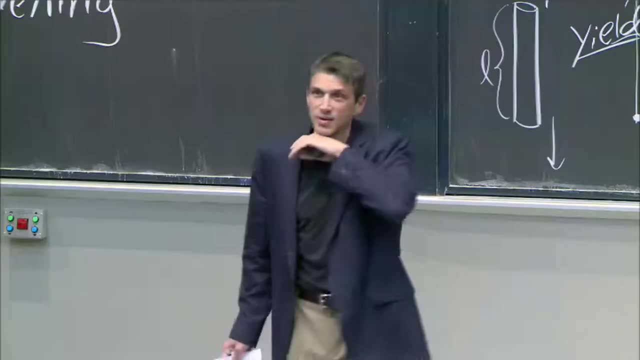 Or is it just going to crack? And, by the way, it's got to have 5 times 10 to the ninth cycles before it can fail. That's like the metric. So that's a pretty big ask of a material. It all comes down to understanding this curve. 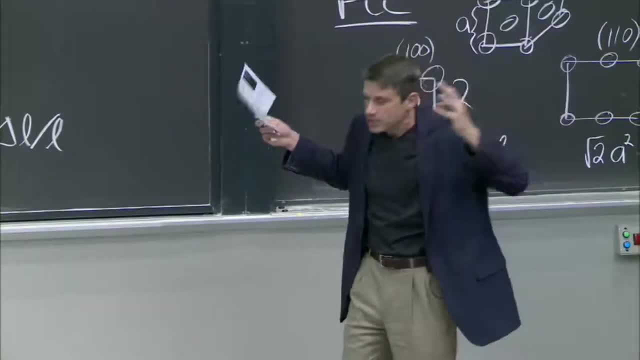 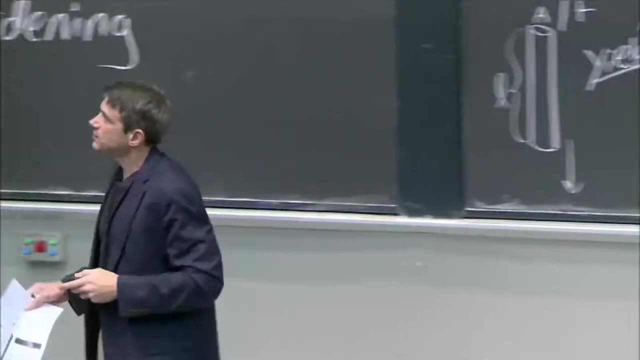 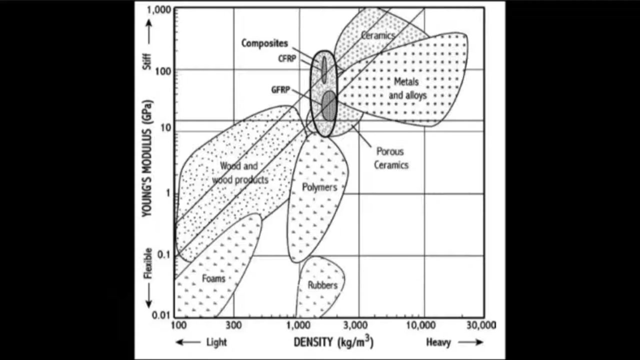 And in the broader sense of materials. this to me is a very exciting ask. Why? Because if you look at a plot of the density of materials- heavy light, good- kilograms per meter cubed And the Young's modulus, now this: 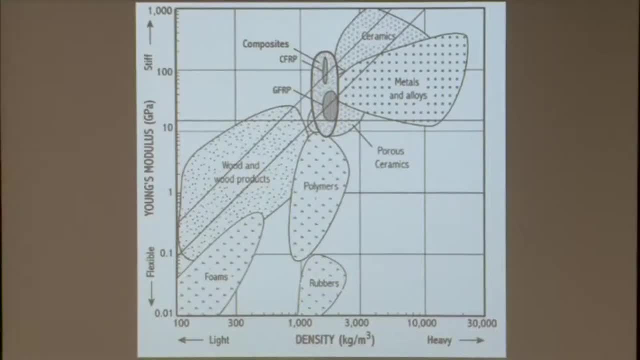 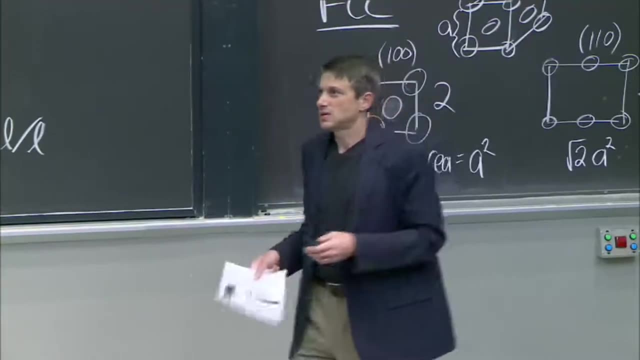 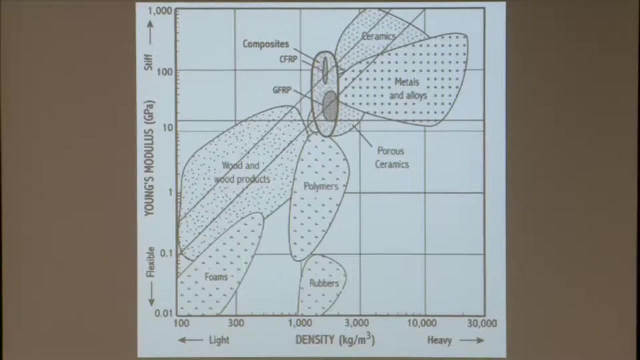 is a measure of the strength of the material. Right, It's a measure of how much strain you could put on the material before it breaks or goes through deformation. But look at this. Different materials are here: Rubbers, foams. OK, foams have relatively low Young's modulus. 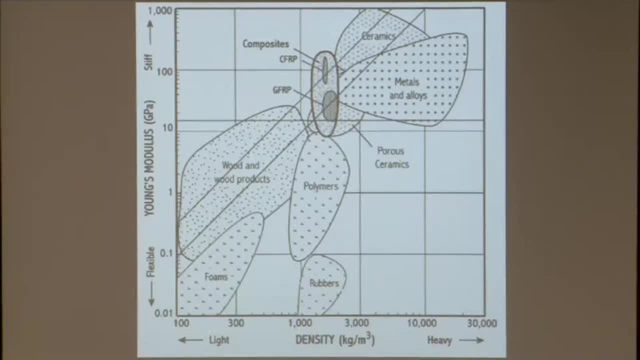 But they're really light. That could be good. Up here you've got metals and alloys, ceramics. You've got polymers in here, But notice, I've got so many different applications And needs in the applications And I've got this plot where I've got nothing here.